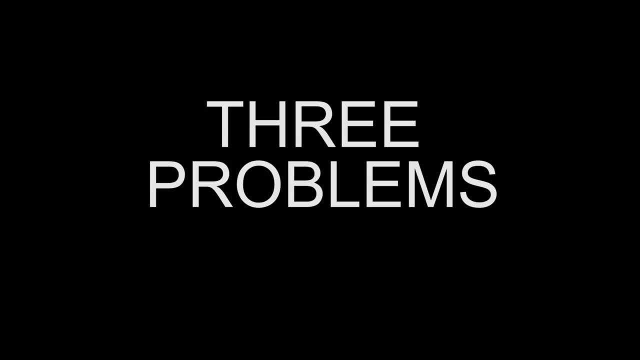 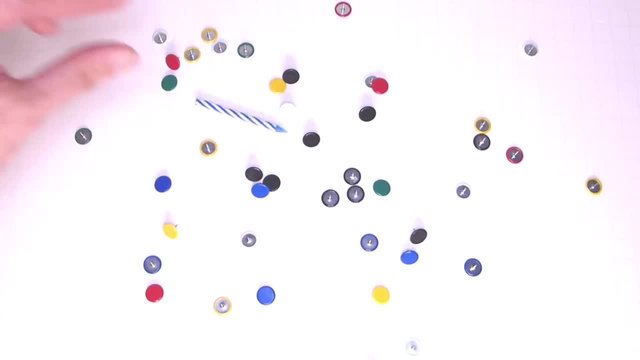 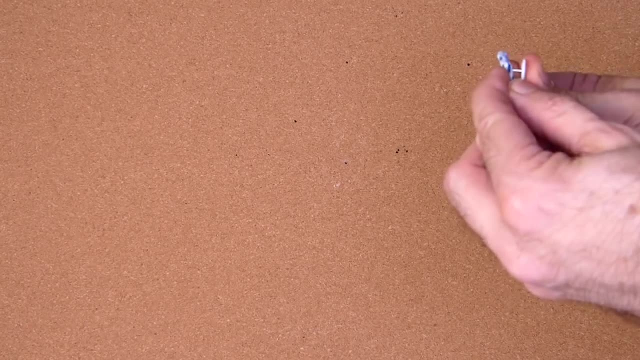 In the candle problem. we're given some thumbtacks, a candle and a box of matches. Don't try this at home without an adult present. The goal state is to attach the candle to a wall in such a way that we can light the candle without burning the house down. 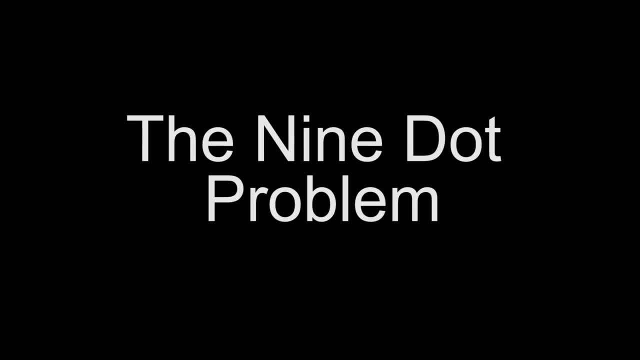 Again. don't try this at home. The nine-digit problem is a problem that we can solve by looking at the problem. The nine-digit problem is a problem that we can solve by looking at the problem. The nine-dot problem was published as a puzzle in the early 1900s. 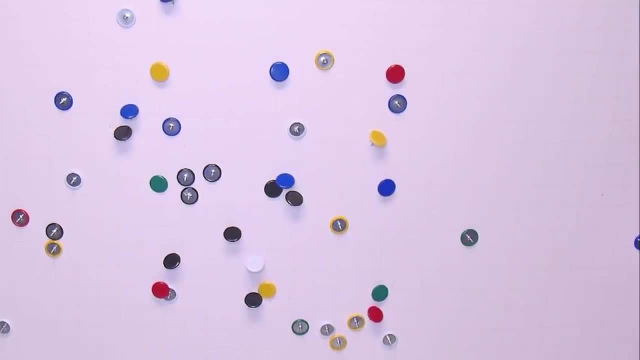 and it seems to have been first studied by the American psychologist Norman Mayer in an article he published in 1930.. The nine-dot problem runs as follows: Given nine dots in three rows of three, connect all the dots drawing through them using only four straight lines. 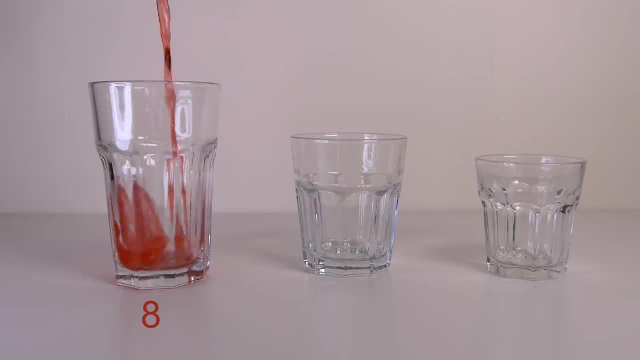 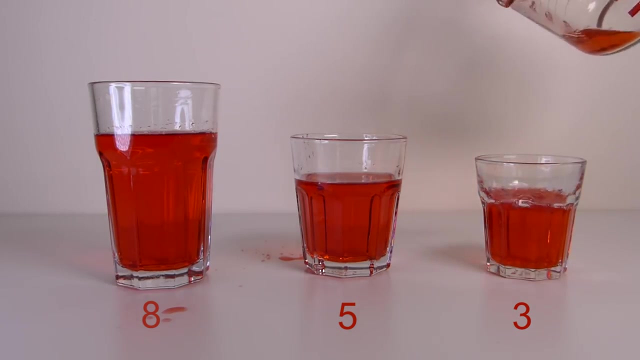 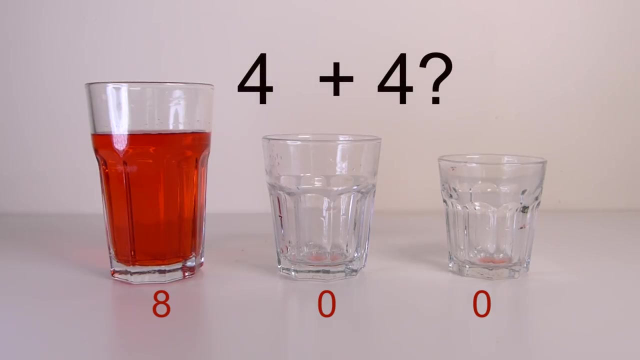 The three-glass problem involves three glasses: An eight-ounce glass, A five-ounce glass And a three-ounce glass. We need to make two servings of exactly four ounces each, without measuring and without just eyeballing or guessing. 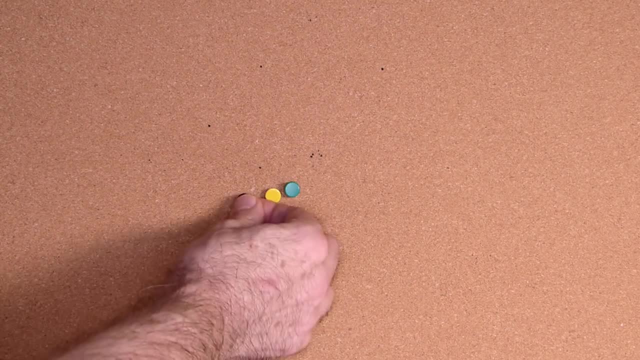 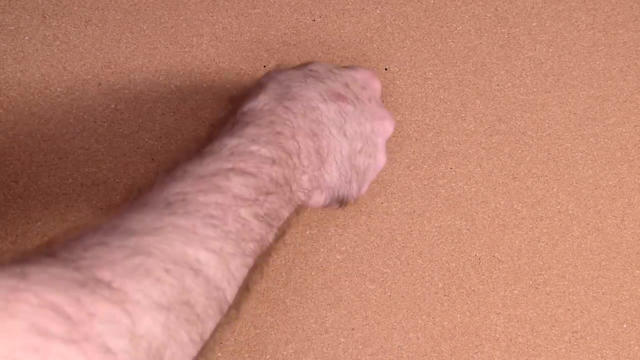 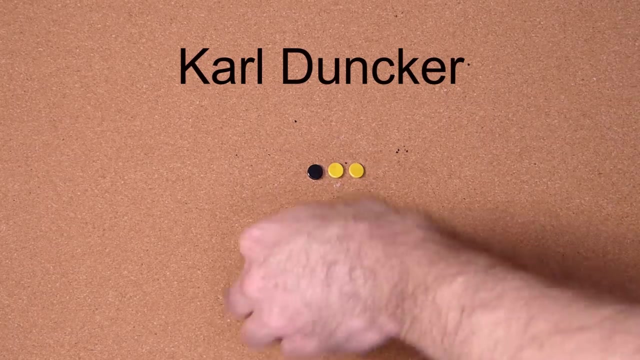 Most people start trying to solve problems using trial and error. This is seldom successful, But it does help you to explore what's called the problem space. The candle problem was the subject of a study by Gestalt psychologist Carl Dunker. In this case the candle is very small, but a bigger candle wouldn't really help. 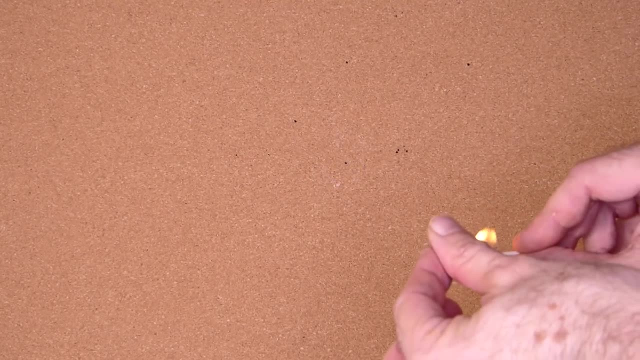 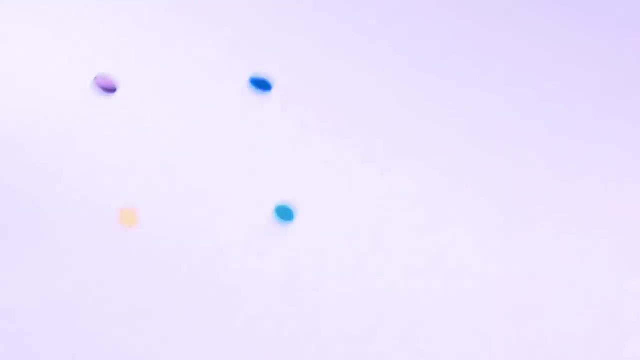 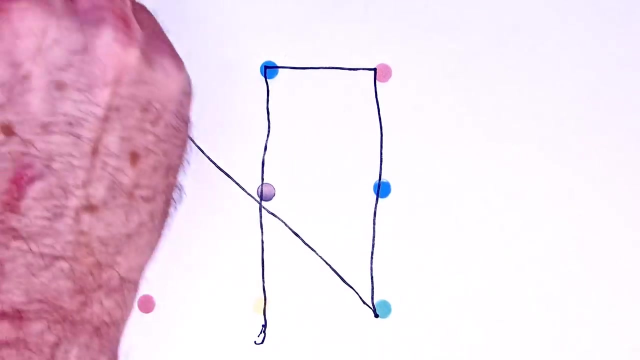 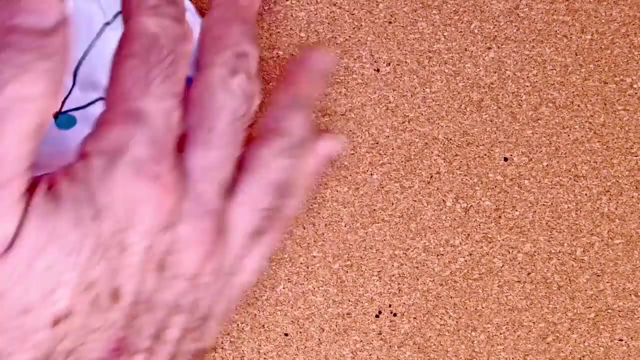 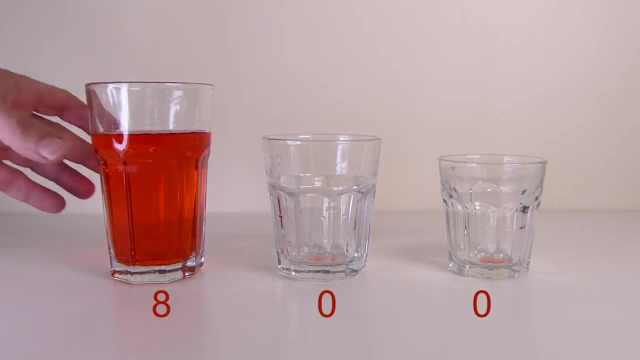 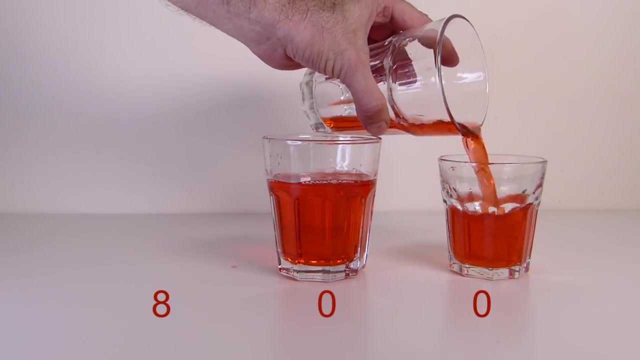 The wax of the candle isn't strong enough to melt it and hold it to the wall. With the nine-dot problem, we can start exploring through trial and error making four lines. Can we run break? It's easy enough to draw four lines, but they don't run through all the dots. 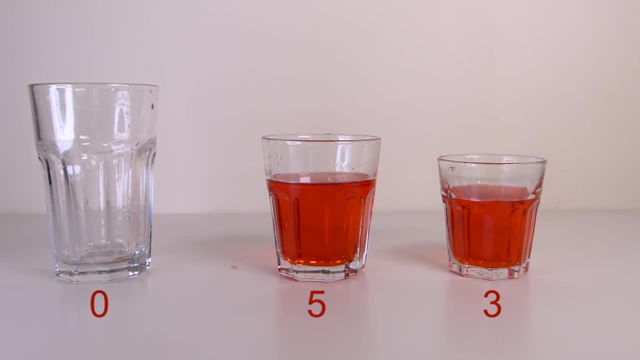 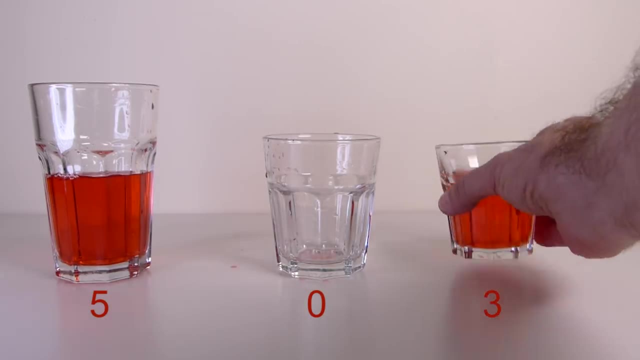 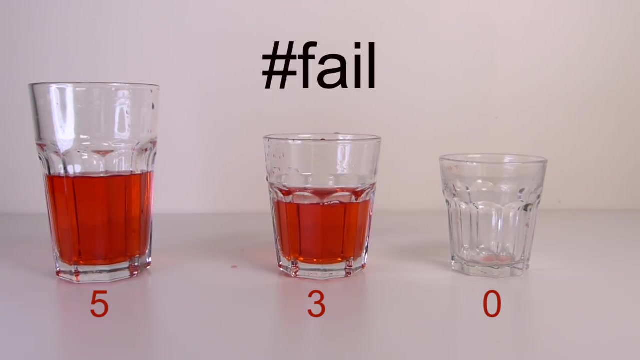 another. We can pour the five ounces back into the eight ounce glass and the three ounces into the five ounce glass, But we basically just keep rearranging five and three ounces in the various glasses. We don't have any way of getting to four. 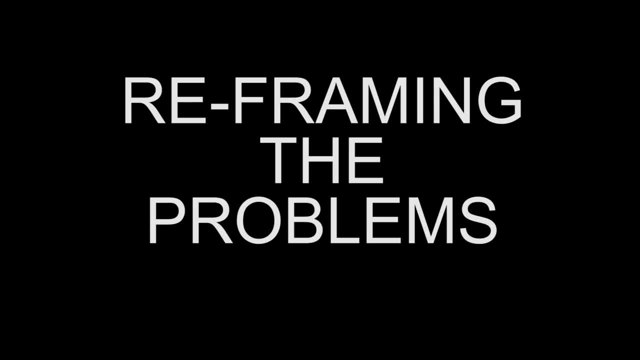 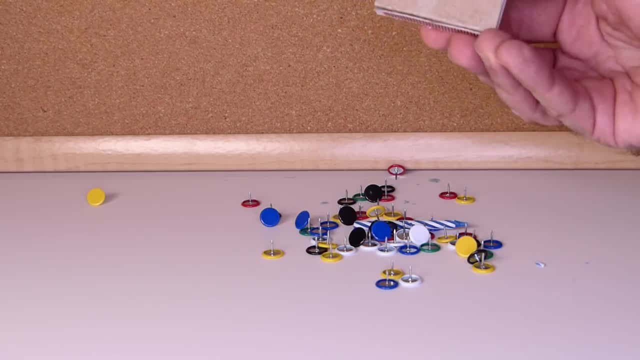 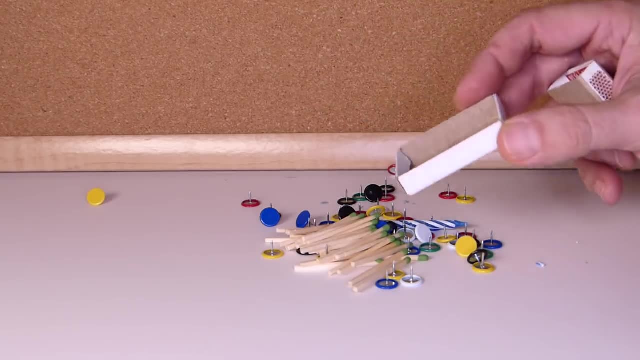 ounces. The solution comes when we realize that the matchbox can be used to make a kind of shelf to hold up the candle. That is, it's not just a box, it's possibly something else. The inability to see the matchbox as a possible solution. 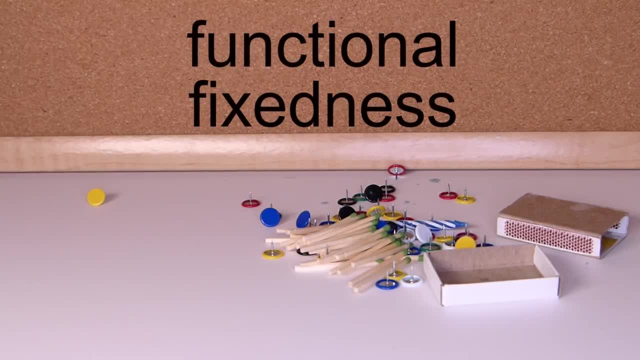 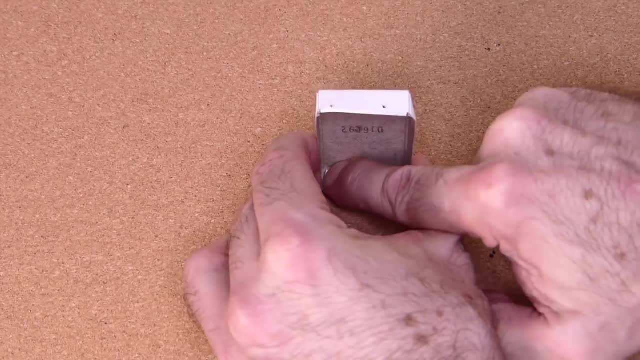 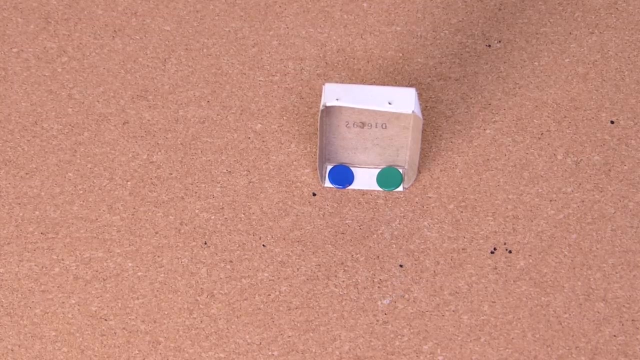 was what Dunker called functional fixedness, seeing an object as only performing one function and not possibly doing something new. Dunker gave his subjects a box of tacks. We're using the box of matches instead. When Dunker presented his research subjects with an empty box and the contents 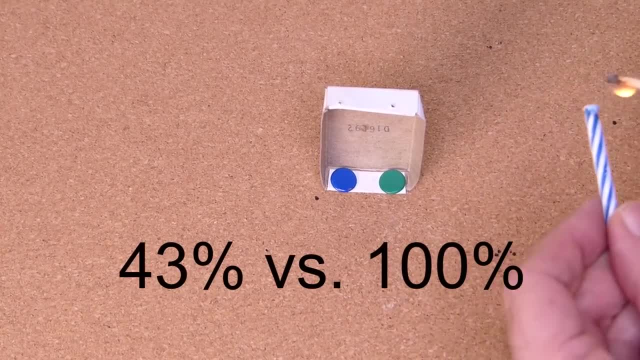 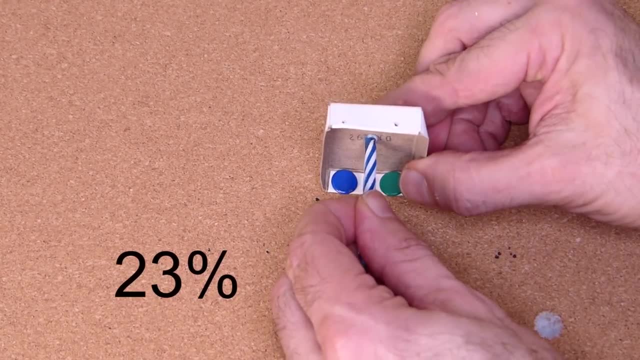 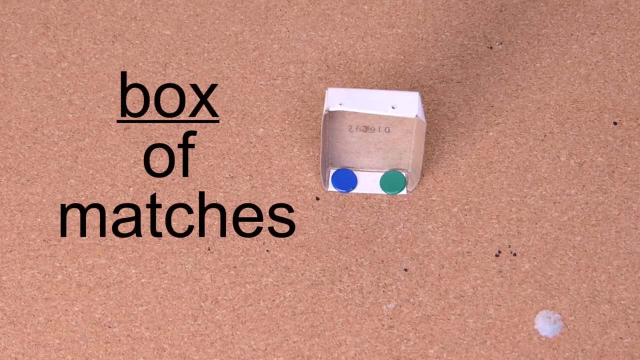 separately, they were twice as likely to be able to solve the problem. Researchers at Stanford found that, solving the problem on paper, about 23 percent of students were able to solve the problem. When the phrase box of matches was underlined, or even just the word box, the success rate rose to 55 percent for 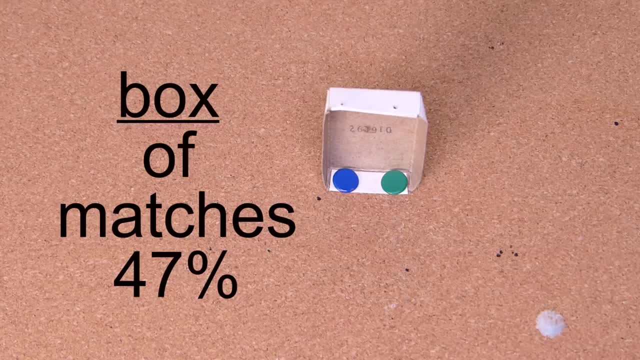 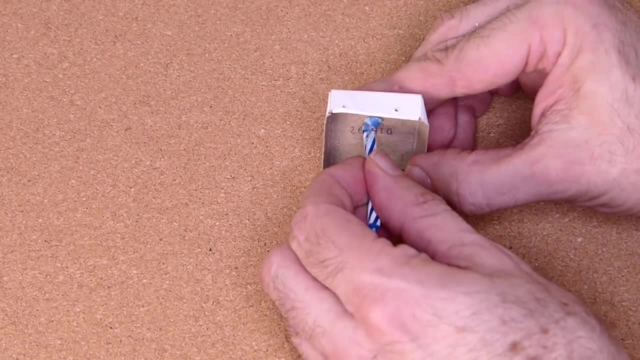 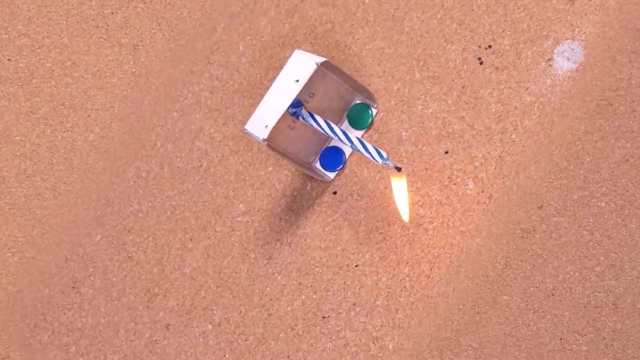 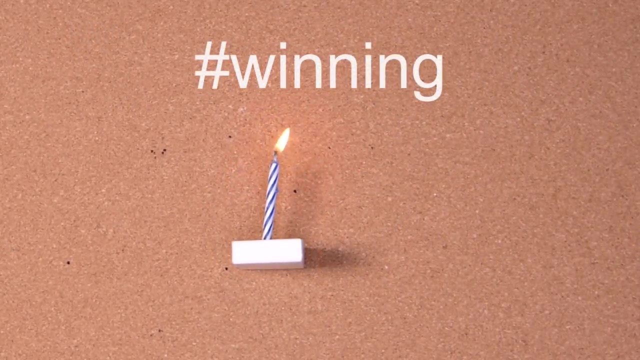 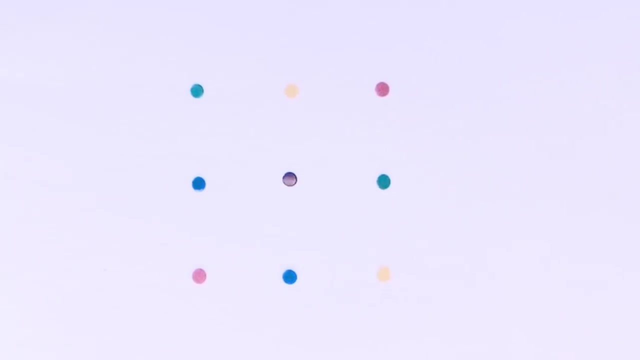 those who had the phrase box of matches underlined and 47 for those who had the word box underlined. The solution comes when we see things in a new way, from a new perspective or angle. One hint psychologists sometimes give test subjects with a nine-dot problem is that it's 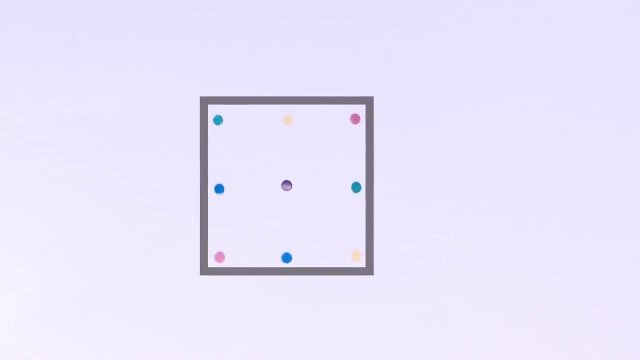 possible to go outside the square represented by the nine dots. If we draw back a bit, we'll get a different view of the problem space. Psychologists still debate today why the nine dot problem is difficult. Some problems are difficult because it's almost impossible to list all the possible solutions or pathways. The nine 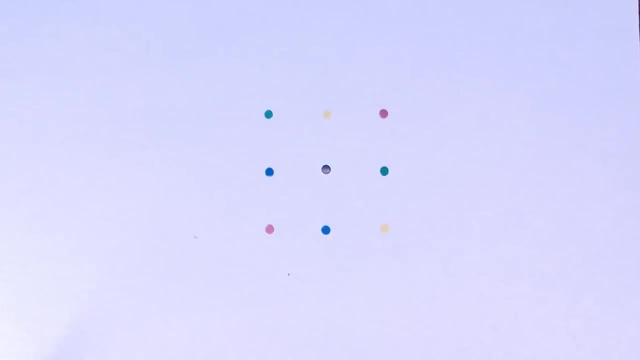 dot problem is not. this way We can explore the problem space by seeing how few lines we can draw that pass through all the dots not worrying about making one connected line. If we do this, there are at least two good ways to use three lines to cut. 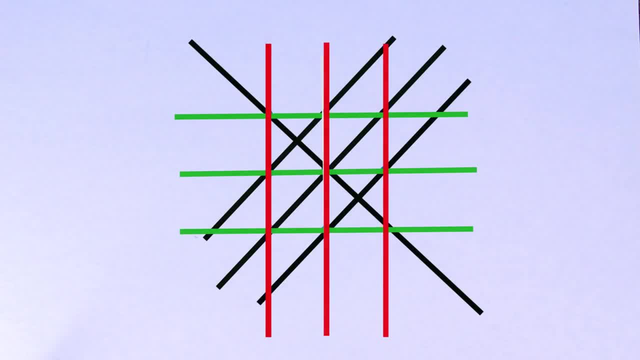 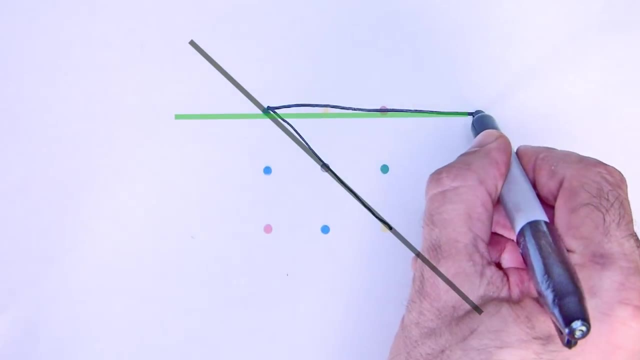 through all the dots and, using diagonal lines, we can do it in four. If we look at this combination of lines, we can realize that four of them will connect outside the space of the nine dots and give us our solution. As with the candle problem, seeing the problem. 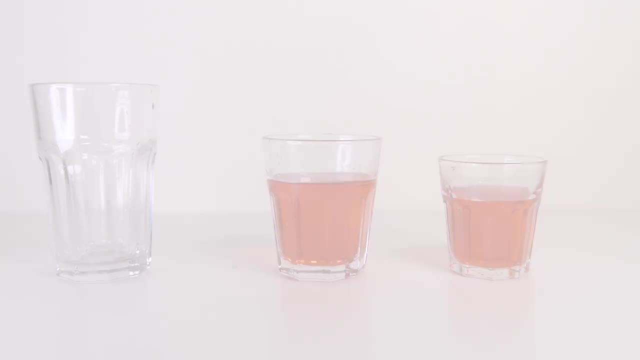 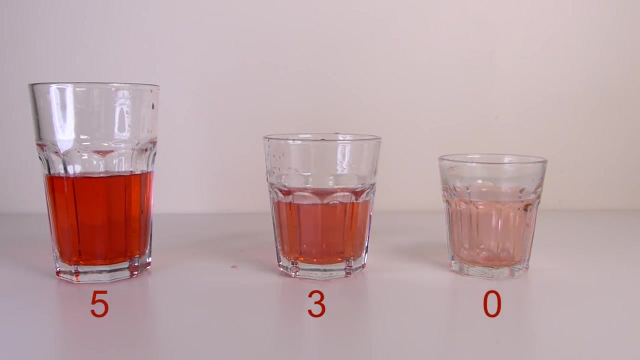 a certain way prevents us from seeing the solution. One problem in our trial-and-error approach to the three-glass problem was we were only thinking about what was in the glasses, not what wasn't in the glasses. If we keep track not only of how much is in the glass but how much extra space is in, 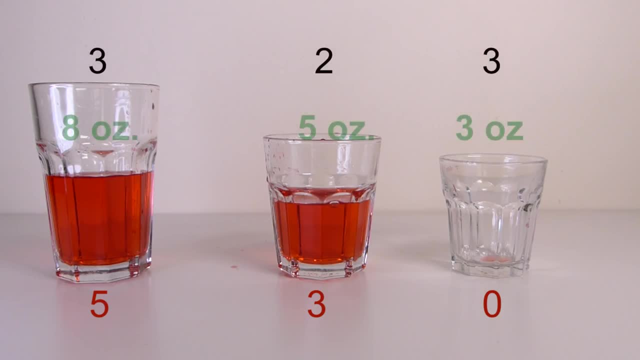 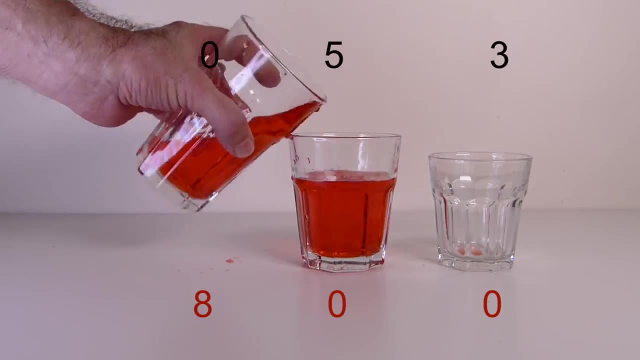 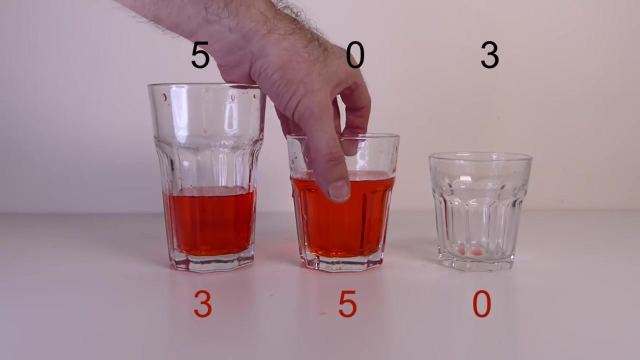 the glass, then we can use that extra space to measure and remove quantities from the other glasses. If we pour five ounces out of the eight-ounce glass, then we have three ounces and five ounces. If we pour liquid from the five-ounce glass into the three-ounce glass, then we end up. 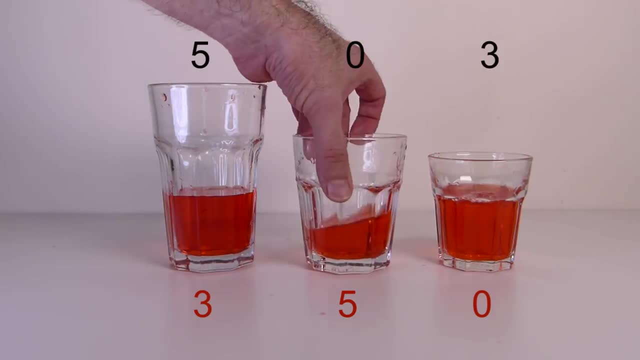 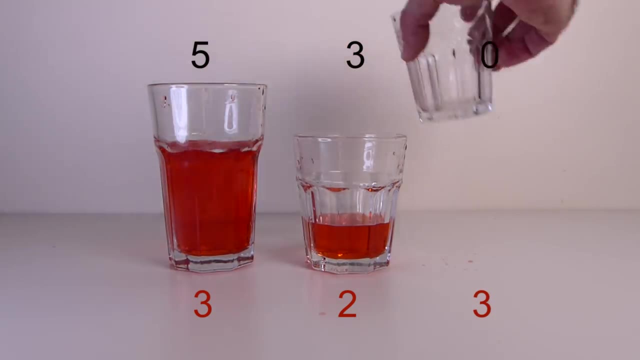 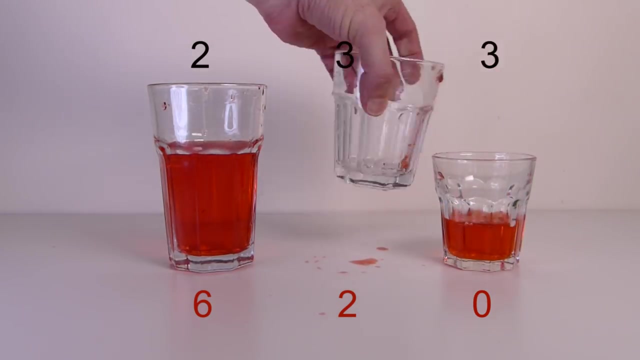 with two ounces left in the five- ounce glass. Combining the three ounces in the large glass and the small glass gives us six ounces in one glass and two ounces in another, which we can rearrange. Now we have one ounce of empty space in the smallest glass. 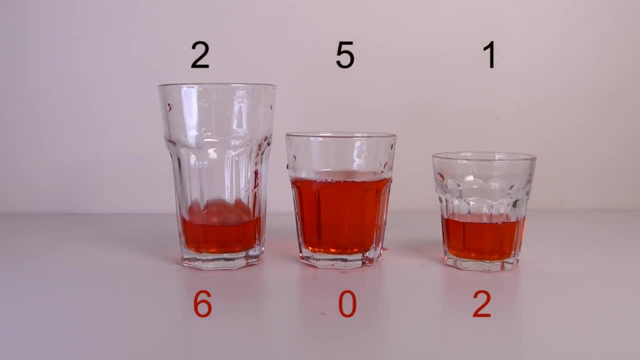 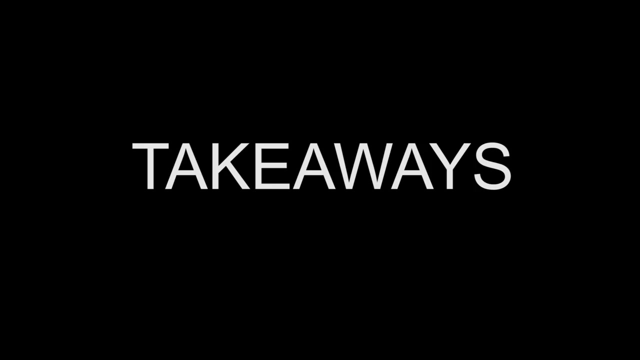 which means if we measure five ounces into the middle glass and pour out some into the three ounce glass, we're left with four ounces. What's left in the other two glasses can be combined and must of course be four ounces. So what does psychology have to tell us about problem solving? Clearly, hints are. 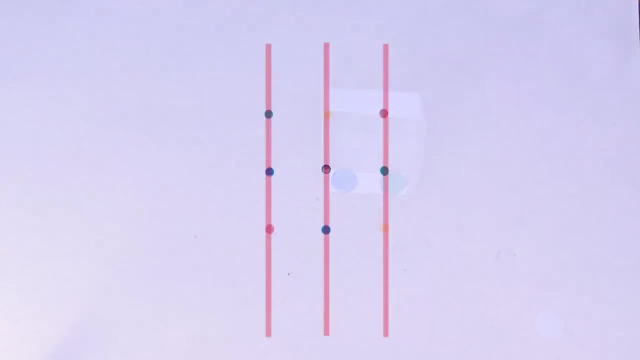 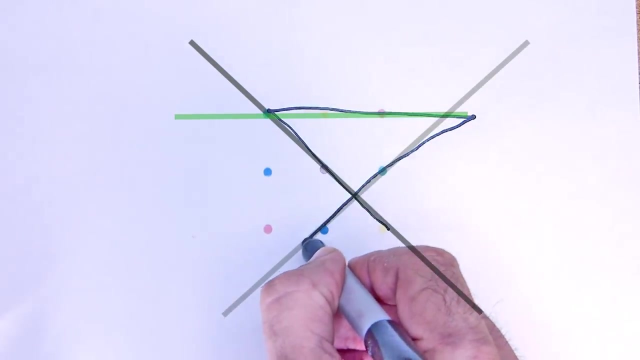 helpful. It's also cheering to know that, by combining elements of solutions that don't work, we can sometimes find a solution that does work. We think inside a frame or box. Indeed, the catchphrase thinking outside the box seems to have come from the nine dot problem. In some cases, we literally need to see what's.